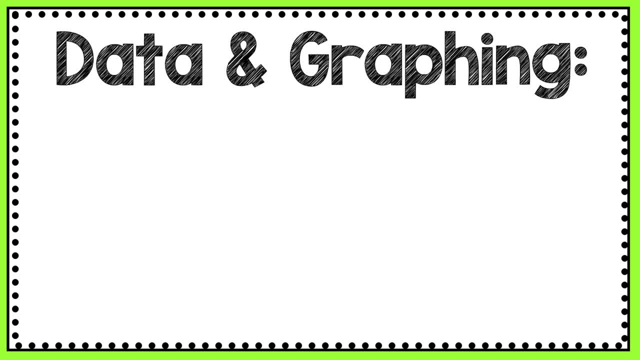 Hello and thank you for watching. Today's video is going to be over data and graphing, but we're going to focus on an introduction to stem and leaf plots. So when I talk about data and graphing, what I'm talking about is information. Data is information and graphing. 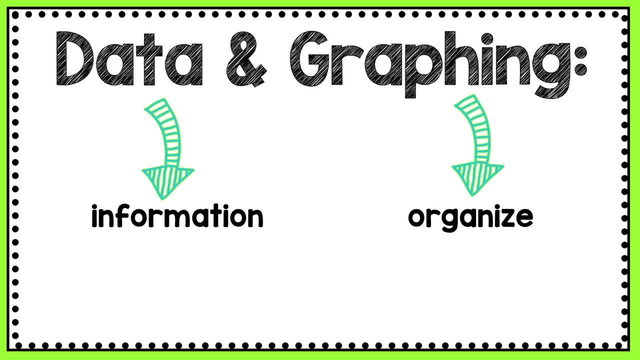 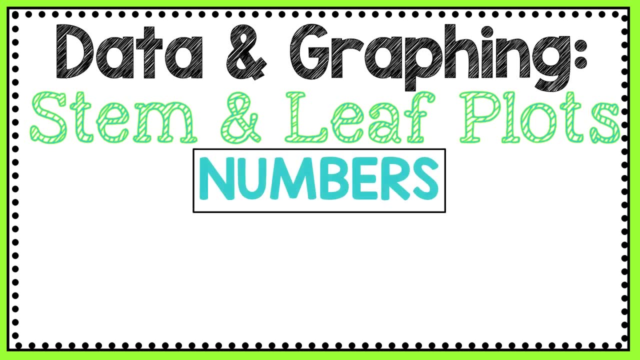 is organizing that information. Now, whenever you're putting math data into a graph, you're putting the information together in an organized way. So let's talk about what you see on stem and leaf plots. You see numbers. That is what stem and leaf plots are for. They graph numbers and you'll see digits like 27,, a two-digit number You may 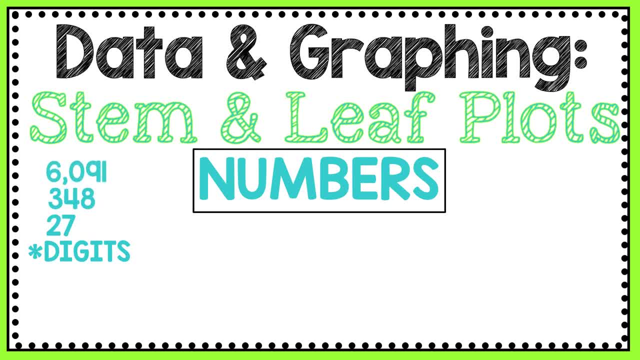 see three-digit numbers like 348 or four-digit numbers like 6091.. So stem and leaf plots, graph numbers. They graph the digits. Stem and leaf plots also graph decimals like 27 hundredths, like a decimal going to the right, like a decimal going to the left, like a decimal going to the. 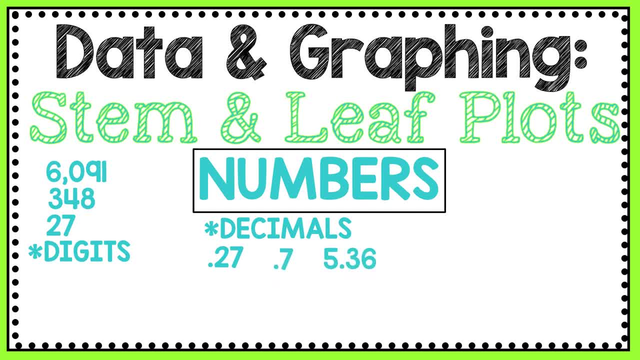 tenths place like seven-tenths and like five and thirty-six hundredths. You can graph those types of decimals And stem and leaf plots. also graph fractions. They can graph just the regular fraction itself with a numerator and denominator, like one-half. You can graph a whole number and 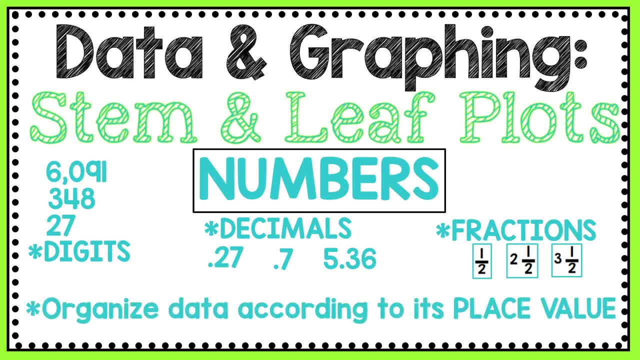 a fraction like two-and-a-half or three-and-a-half. So the main thing you need to remember about stem and leaf plots is that they organize data according to a number's place value. So the main thing you need to remember about stem and leaf plots is that they organize data according to a number's place value. 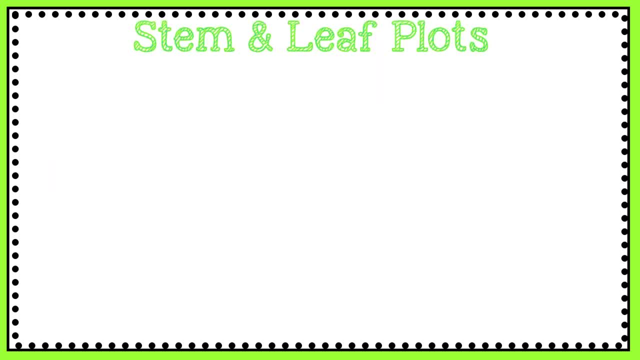 So let's look at some stem and leaf plots. This is what a stem and leaf plot looks like. It looks like a T chart and you graph a number's place value on the T chart. Now, on the left you'll see the stem and on the right you'll see the leaf, and that won't change The stem. 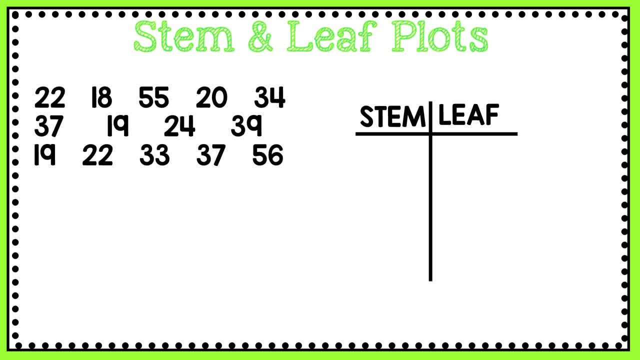 and leaf always stay in the same place, So let's graph some numbers. Now. here I have a set of data and I want to put these two-digit numbers on my stem and leaf plots. now, an important rule whenever you're graphing stem and leaf plots is that you want to put the 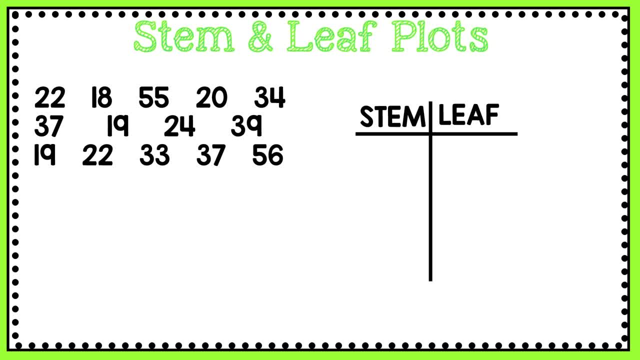 numbers in order from least to greatest, because stem and leaf plots order numbers from least to greatest going this way, and the number that has the least value starts on this first row and then goes to the greater value down this way. so that is how stem and leaf plots graph numbers. so I'm 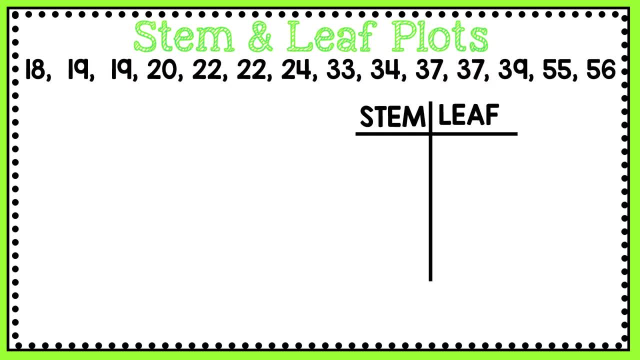 going to put these numbers in order from least to greatest. so here's my list of numbers already, in order from least to greatest. this is gonna make it much easier to put on my stem and leaf plot. and before I move on to put them on the stem and leaf plot, I need to look at the key now. remember I said: 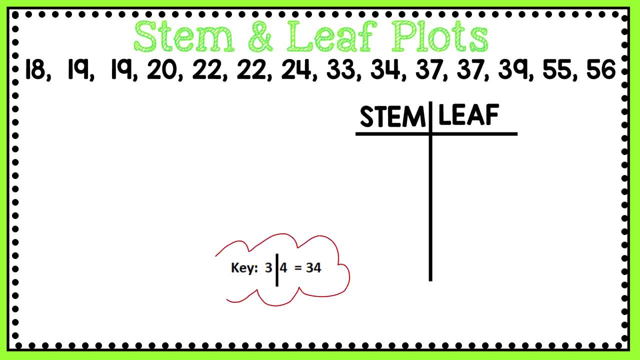 in my other videos. the key is very, very important. it's going to tell you what the numbers mean on the stem and leaf plot. so in this case, my key tells me that if I have a digit in the stem, like the three, and a digit in the leaf, like the four, I'm going to be plotting a two digit number, like 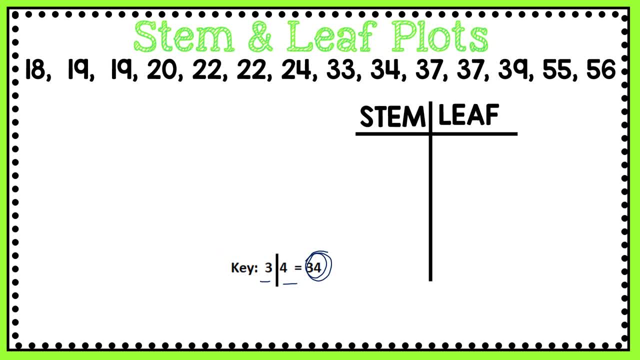 the three and a digit in the leaf, like the four. I'm going to be plotting a two digit number, like the number thirty four. now, this is going to be a fairly easy stem and leaf plot because we're plotting two digit numbers. so let's take my first number, eighteen, and to represent eighteen on the 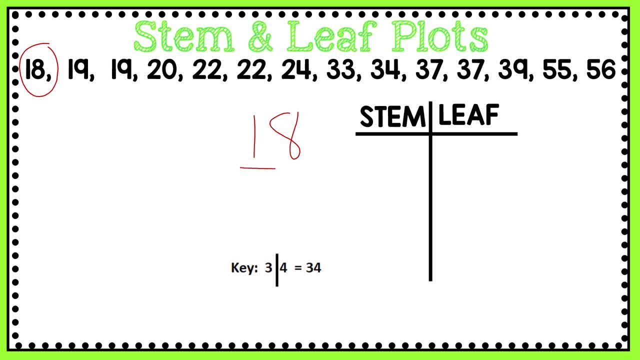 stem and leaf plot. I look at the first digit in the tens place. it is a one. so one will be my stem and eight will be my leaf. so one eight in the stem and leaf plot represents eighteen. I've graphed that. I'm going to cross it off. now let's look at the next two I have 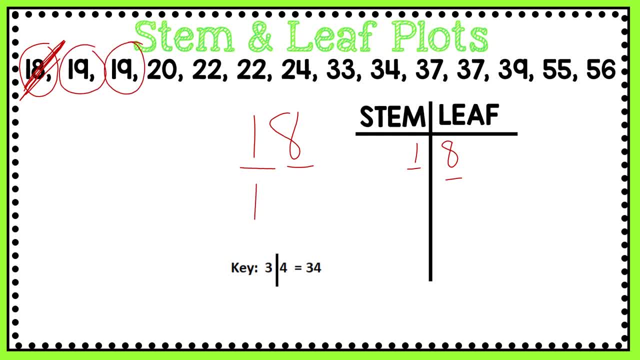 nineteen and nineteen, so to represent nineteen. the one in the tens place is already in the stem, I don't have to put that again, it's already there. so I'll take my nine and I'll place it in the leaf. so this one and this nine represent nineteen, and then I have another nineteen, so I need to. 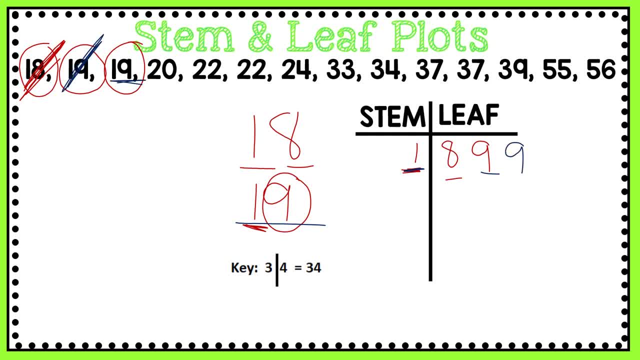 represent that one. so I will take my nine and put it in the leaf. and now I've represented 18, 19 and 19. now let's go to my next number. the next number I have is 20. now I have a 2 in the tens place of. 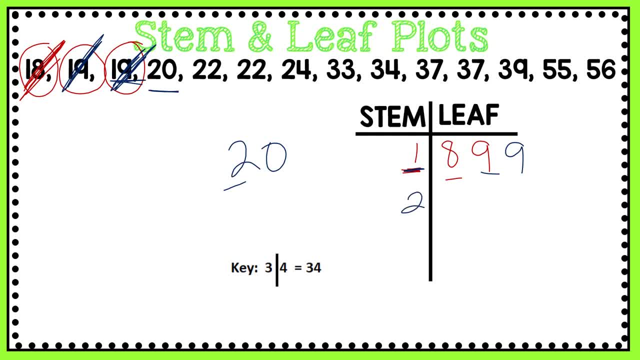 my 20, so 2 will be my stem. now notice I'm starting a second row here to represent the numbers with 2 in the tens place. so 2 will be my stem. so the 0 goes in the leaf and the 2: 0 represents 20. then 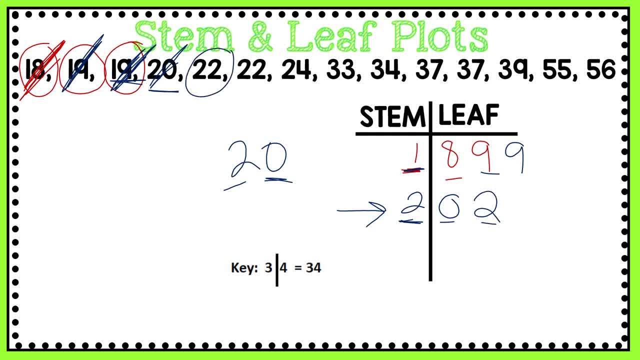 we'll put a 2 in the leaf and that represents 22. I have another 22 here and I'll put my 2 in the leaf there, so that represents another 22. and then I have a 24, so 24 will go on the leaf side. 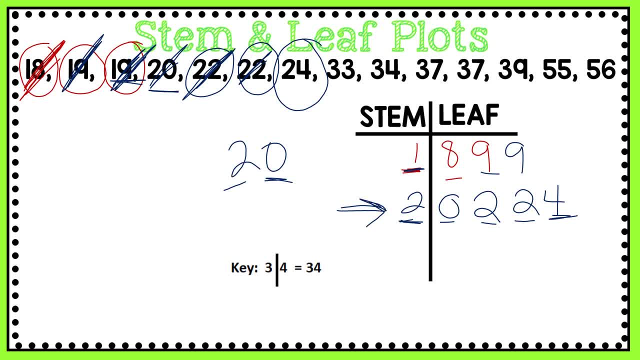 with a 4, and this row represents numbers with a 2 in the stem. so now I'll start another row with numbers that have a 3 in the stem, because I have numbers in the 30s. so my new row will have a 3. that represents my numbers that have a 3 in the tens place. like 33, I have a. 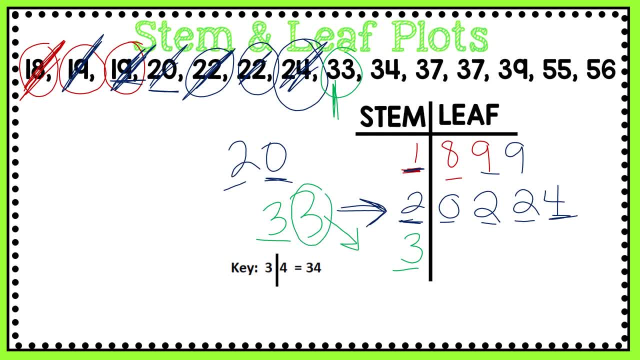 3 in my tens in my stem, and the 3 in the ones place will go here in my leaf, so that's 33. next I see I have 34. I will put a 4 in the leaf, then 37. I will put a 7 in the leaf representing 37. 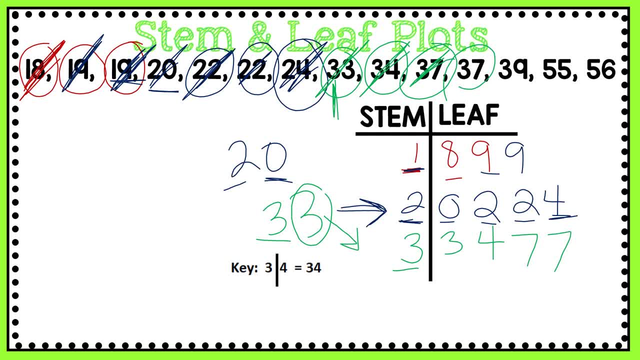 and I have another 37, so I'll put another 7 there and then 39, so the 9 in the leaf represents 39. I have one more row of numbers and those are the numbers in the 50s, so I will put my 5 here in my stem. and sometimes you need to make your 7 leaf plot. 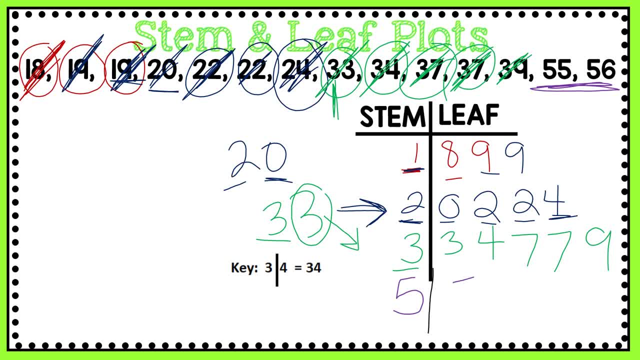 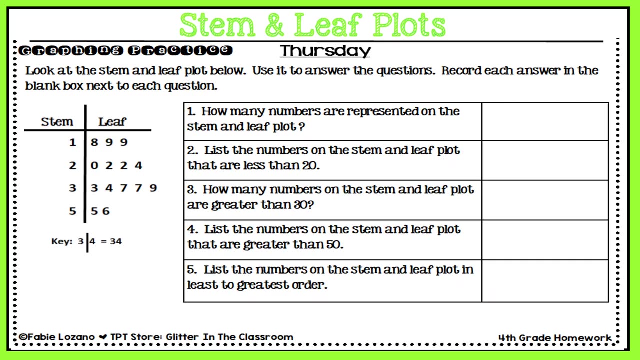 a little longer, that's okay. and the 5 in the leaf represents 55, and I have 56, my last number to go in my stem and leaf plot. this 6 goes in the leaf and that represents 56. so this is how to take numbers: take a data set like this and place this inside of a stem and leaf plot. now 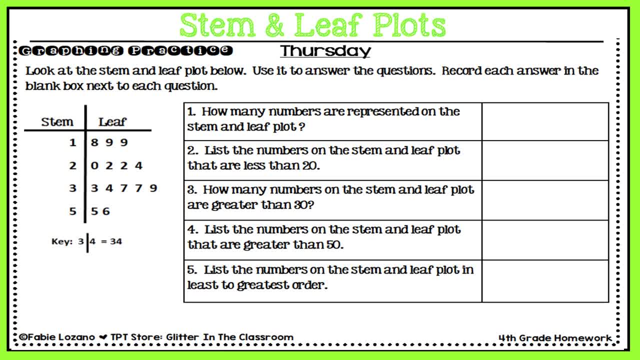 let's answer some questions on the stem and leaf plot that we just did. as you can see, the stem and leaf plot that I put together on the previous screen is right here now. it says: look at the stem and leaf plot below. use it to answer the questions. record each answer in the blank box next to each. 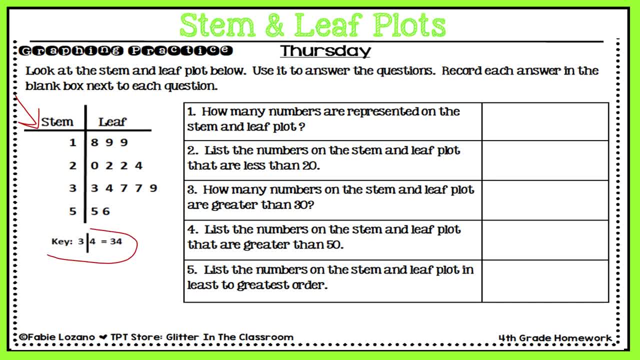 question. so here's your stem and leaf plot. here is the key, same key as before, and I know that these are two digit numbers because my key tells me that the stem and leaf plot is equaling to two digit numbers. so let's look at number one: how many numbers are represented on the stem and 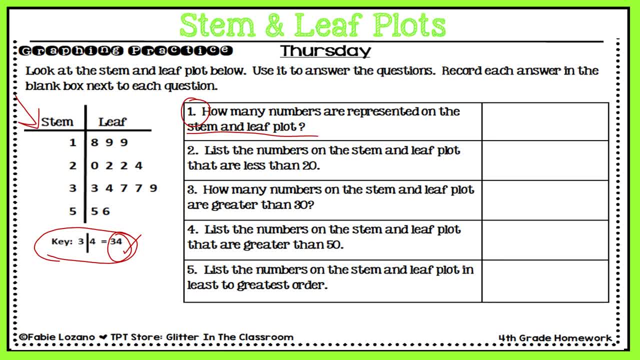 leaf plot. now, this is a fairly easy question because all it takes is for my eyes to look and observe the leaf side. so I see that I have 1, 2, 3, 4, 5, 6, 7, 8, 9, 10, 11, 12, 13, 14 numbers represented. 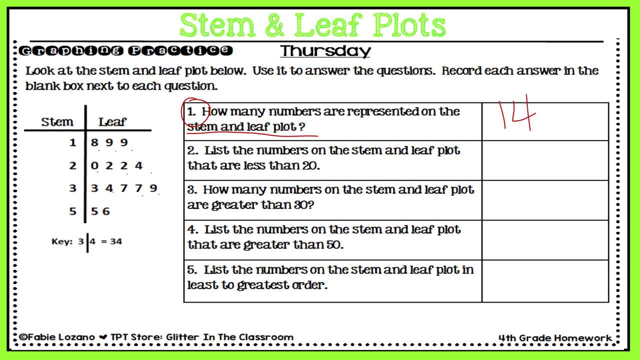 on my stem and leaf plot and, if you remember from before, we listed those numbers in an order from greatest to least. so if I needed to, I could just count the list that I had. now let's look at number two list, the numbers on the stem and leaf plot that are less than 20. so I have to go to my stem and leaf plot now, remember. 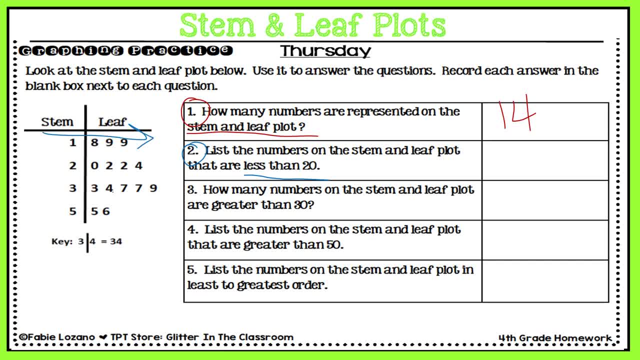 I told you, it's an order from least to greatest going this way and least to greatest going this way. so it's pretty easy, once it's organized, to find numbers that are less than 20. so I'm going to go to my stem and leaf plot that are less than 20. so here is 20. but I do not want 20, I want the. 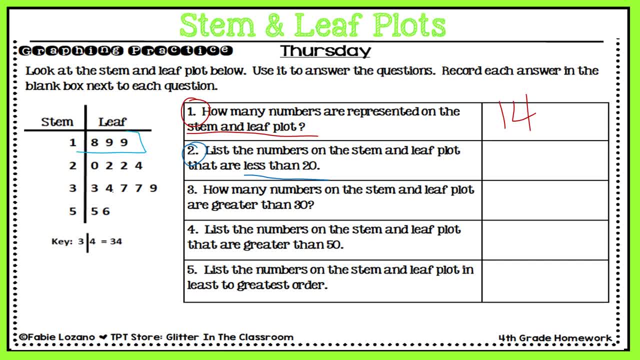 numbers that are less than 20, and that would be these numbers here: 18, 19 and 19.. so it's asking me to list them, and the numbers on this stem and leaf plot that are less than 20 are 18, 19 and 19.. 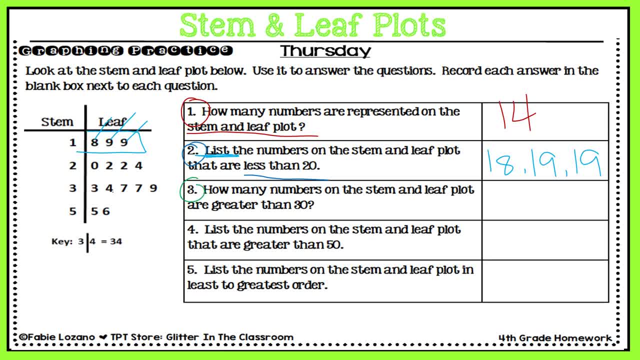 let's go to number three. how many numbers on the stem and leaf plot are greater than 30. so I will not be including 30. I need greater than 30. and I like to put brackets on these ones, so I'm going to go ahead and put a bracket here. I know that the numbers greater than 30 are there and it ends here. 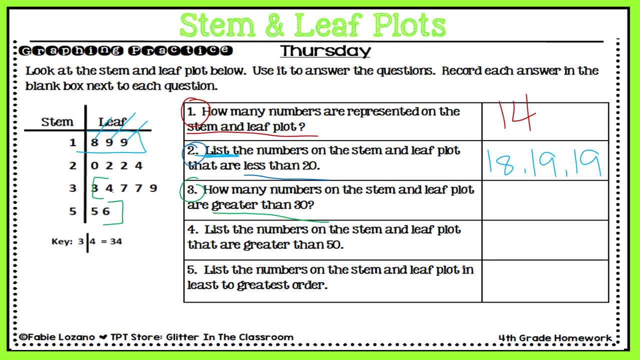 so how many numbers are greater than 30? well, let's count one, two, three, four, five, six, seven, seven numbers are greater than 30.. so let's go to the next question. number four: list the numbers on the stem and leaf plot that are greater than 50.. I'm looking for numbers that.